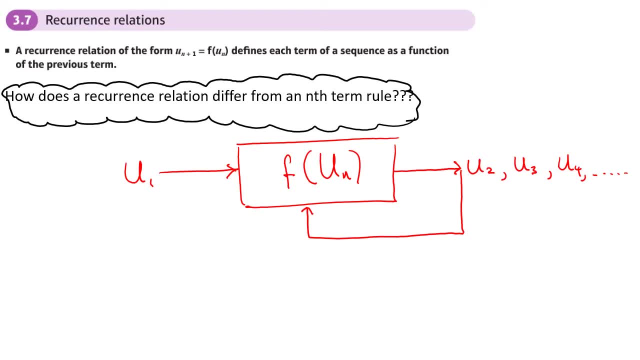 term number in to get the term with a recurrence relation. you put the last number in to get the the next term, so you always need the last one to get the next one. now, sometimes when we write a recurrence relation out, it is possible to convert it into an nth term rule, because you might see 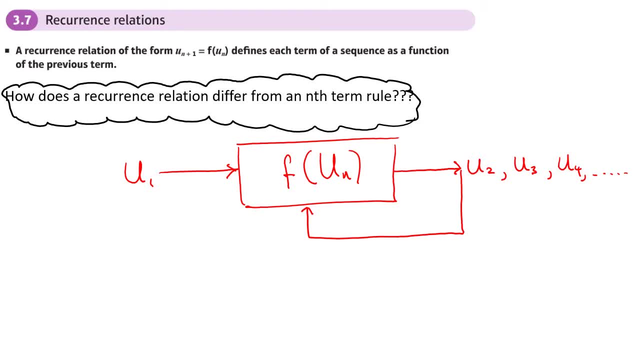 a pattern or for an arithmetic sequence or a geometric sequence. so actually what we might find is: this recurrence relation produces an arithmetic sequence or a geometric sequence. that's possible, sometimes it doesn't. it may produce a nice pattern, but it may not necessarily be a pattern that we can write a rule for. it all depends. 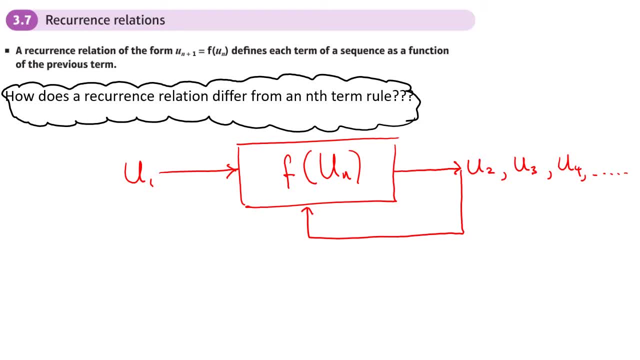 on it now whenever um the next number comes out here. i suppose what we could do is we say that we get up to um. the next term is always going to be un plus one, so i'll just rub those out to give myself a bit of space. 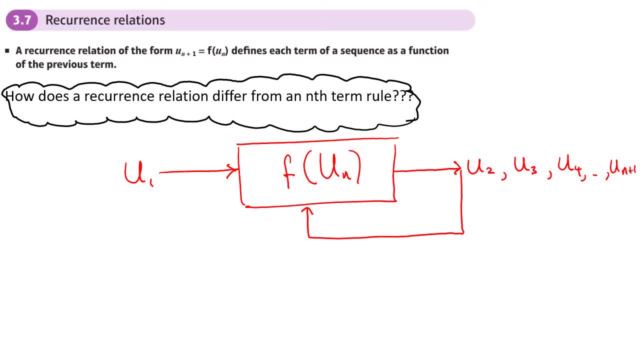 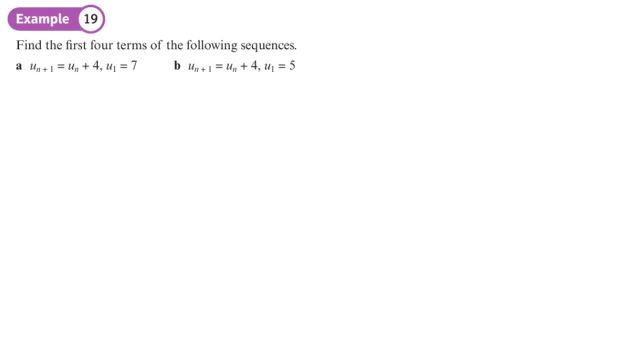 so u n plus one is going in in general is the next term. yeah, here we're just asked to write out the first four terms of the following sequences, so you can see you're giving the starting value and you're given the rule. so you have to work out. 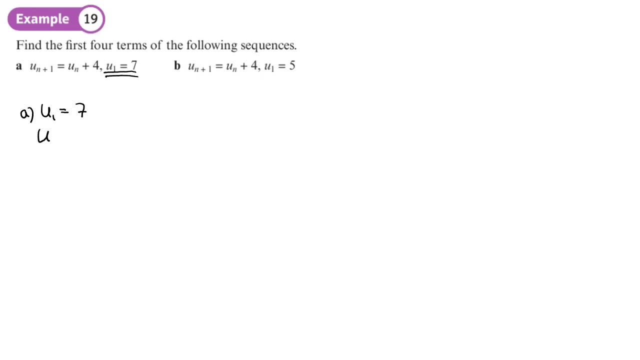 one at a time. so u1 is seven, that's given u2. well, you take u1 and you add out four to it, so it's going to be the last term, i2 plus 4, which is 11.. u3- well, that'senn keyword 4. 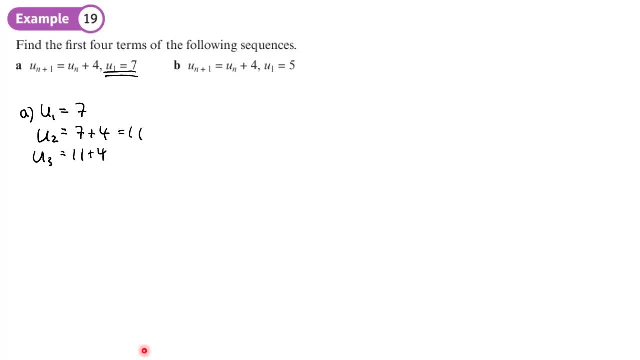 just going to be the last term: 11 plus 4. so you can see the rule up here. it basically just says: take the last term and add 4 to it is 15 and u4 that's going to be 15 plus 4- 19. so there we go. the first four terms: 7, 11, 15 and 19- 7- 11. 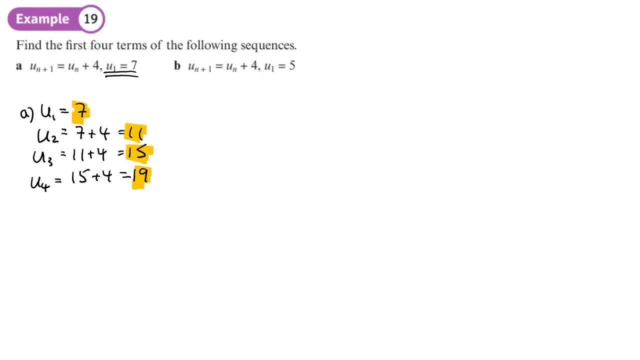 15, 19, part being slightly different rule, different starting number. so this time you 1 is 5 and it's the same rule as the last one. it's taking the last number and adding 4 to it, so it's going to be 9 u 3 is going to be 9 plus 4: 13 u 4 is. 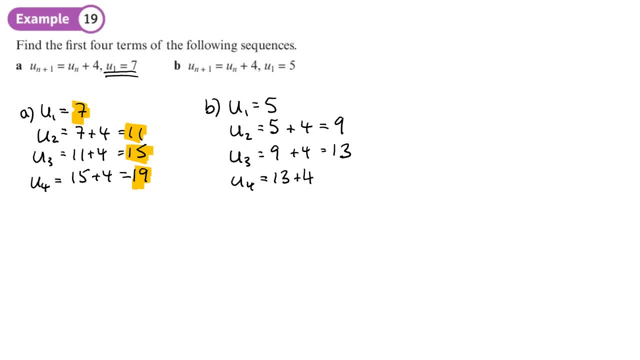 going to be 13 plus 4. so because we have a different starting number, our our sequence is going to be 13 plus 4. so that's going to be 13 plus 4. so, because we have a different starting number, our sequence is slightly different to the last one, in that it it's just too lower because the 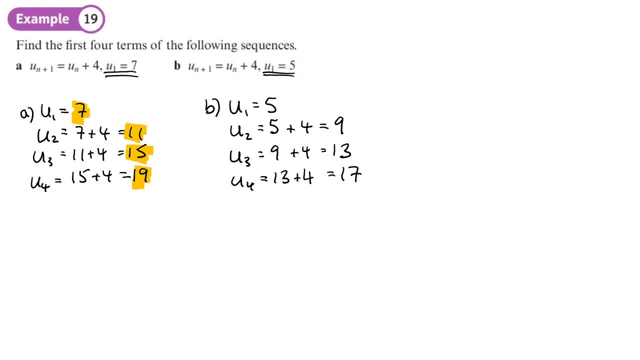 starting number was too lower than that one. okay, nice, easy, basic stuff: 5, 9, 13, 17. so here what we have is some information. we're given the first term and it's given algebraically as P and we're given the rule here. here is our, our roll, and there's some information about P and n. n is greater. 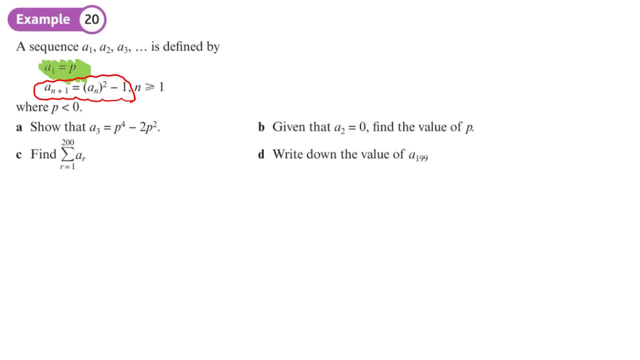 than equal to 1. P is less than 0, so that might tell us something about our solutions. and it says: showed that a 3 is that expression right? well, we'll start with a 1 which we're given, which is P, now together to: I plug this into the: 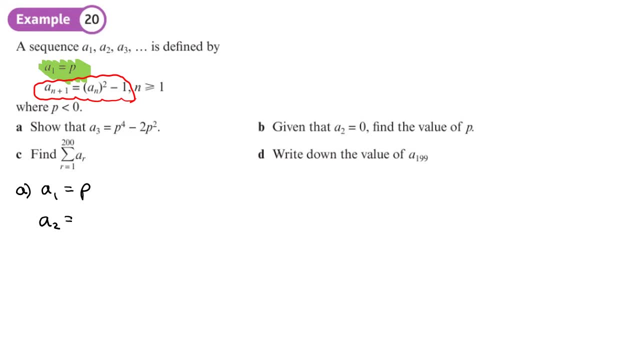 recurrence relation. so that's going to be a 1 squared. so P squared, my 수도2.b f2 equals薠 1. then I take that and put it in again. so a 3 is going to be the last value squared. so that's P squared minus 1. squared minus 1. it's just given in a. 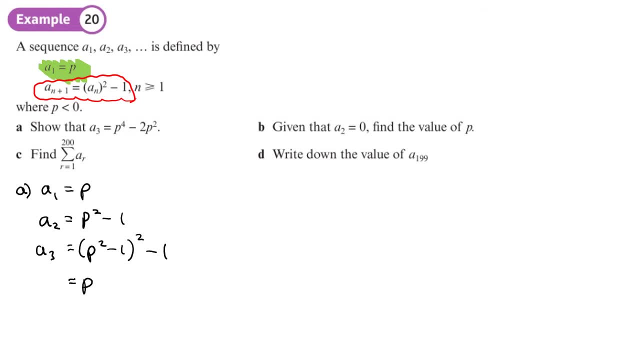 different form, so I'm just going to expand the brackets so that'll be P to the power 4 minus P squared minus P squared plus 1 minus 1. so yeah, I can see I'll get P to the power 4 minus 2 P squared. QED right part B, given that a 2. 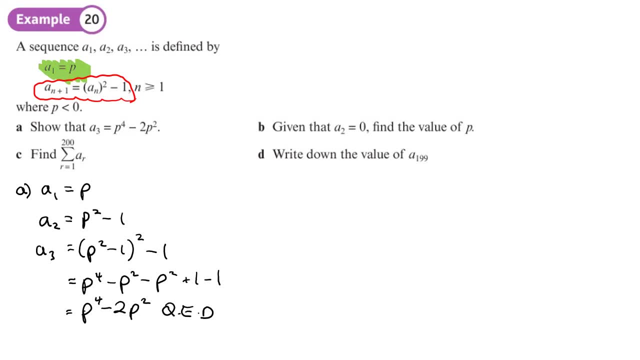 equals 0. find the value of P right. a 2 is this one, and we're told that that equals 0. so that means that P squared minus 1 equals 0, which is P squared equals 1. now P could be at plus or minus the square root of 1, but up here it said: 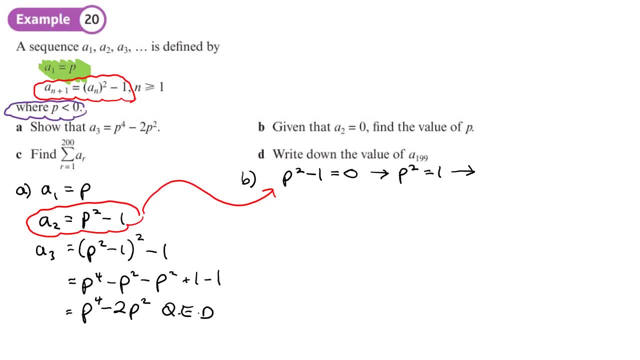 that P is less than 0. so actually we'll write down that P is plus or minus 1, but then we'll say: since P is less than 0, P equals negative 1. so that piece of information was there for a reason. okay, part C, part C: find the sum of these 200 terms of AR. so we're going from R. 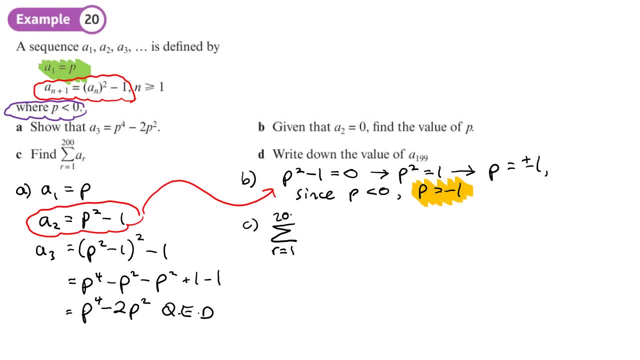 equals 1 to 200. now, since we've already worked out the value of P, we can actually- you know, I said that we'd normally use this to write out the first three terms. well, we've got the first three terms over here, so let's just. 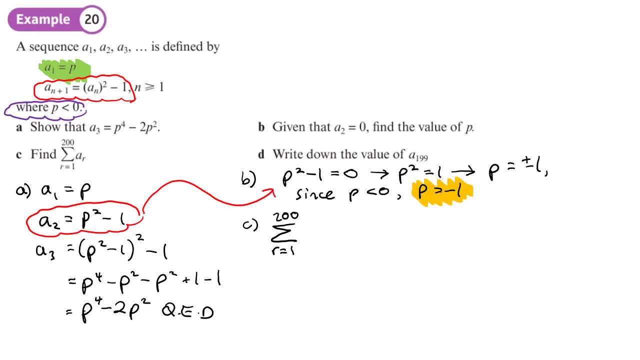 write a negative 1 in and see what we get for the first few terms, and we can use that to help us decide where this arithmetic geometric, what the first term is, what the common difference or common ratio is, how many terms, well, terms of 200, right, so a 1. the first term is going to be negative. 1 because P is negative. 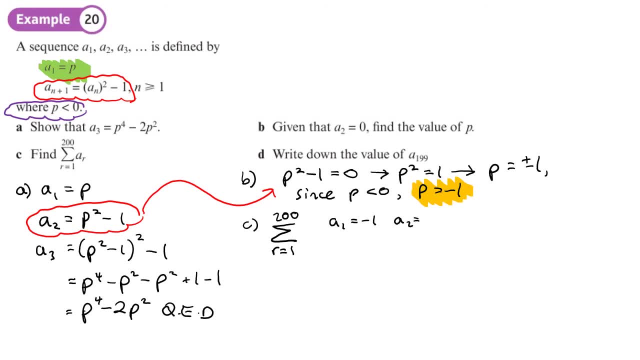 1. a 2, the second term. well, that's just going to be negative 1 squared minus 1. and well, actually we're told that it's 0, isn't it? and then the third term, a 3. well, that's going to be negative 1 to the power, 4 minus 2 times negative 1. 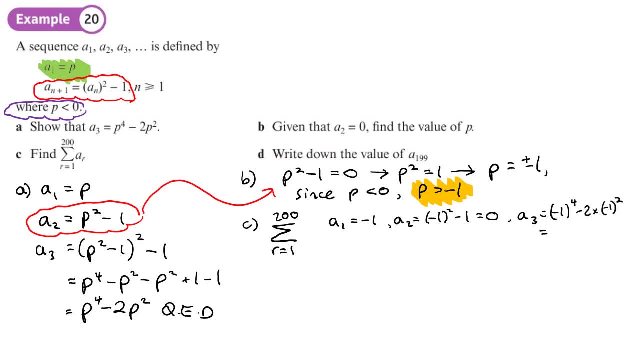 squared, so that is going to be 1 minus 2, which is going to give you negative 1. now it looks like this sequence is going: negative 1, 0, negative 1. it looks like it's this what we call periodic pattern. now, just to check that, I'm actually going to work out what a 4 is and I'm 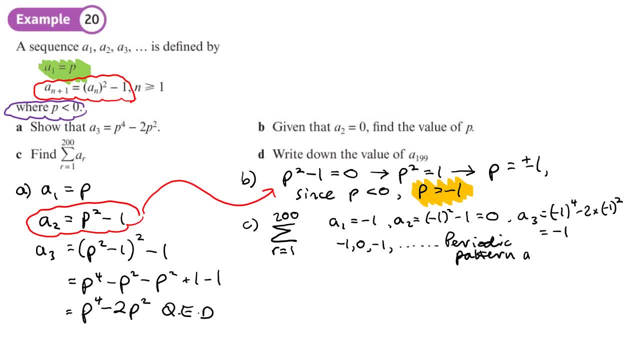 expecting a 4 to be 0. now, this will require a little bit of work. so a 4, not a, to the power: 4, a 4. that's going to be our last. a 3 squared, so I can just now put the numbers in. so a 3 squared, which is negative, 1 for a 4 minus 1, so that's. 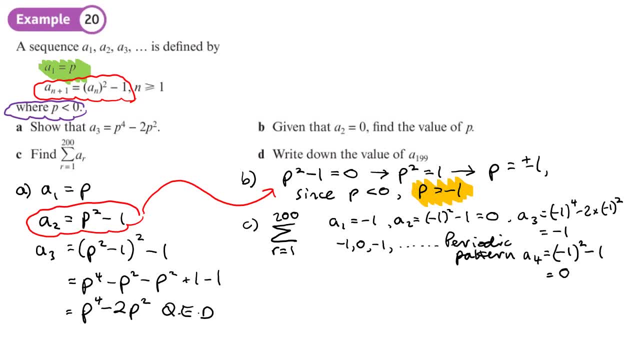 going to be 1 minus 1, 0, then the next one is going to be that squared minus 1. so it is a periodic pattern that goes like that and in fact I could have saved myself a bit of time and I could have actually just put the number straight. 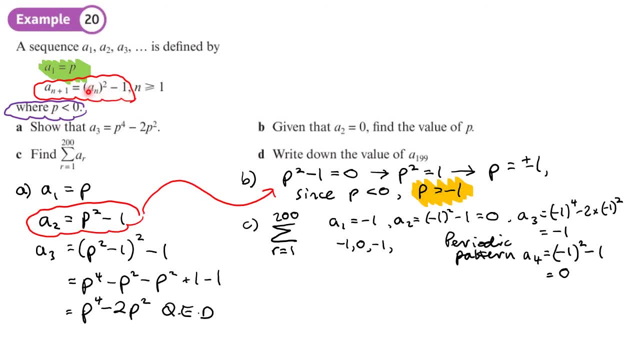 into there? yeah, because the next term is just the last term squared minus one, so I could have saved some time there. surprised I said anything right, so if I'm adding up these 200 terms, it's actually going to be. it's not geometric and it's not arithmetic, is this? it's this pattern. now, what am I going to have? 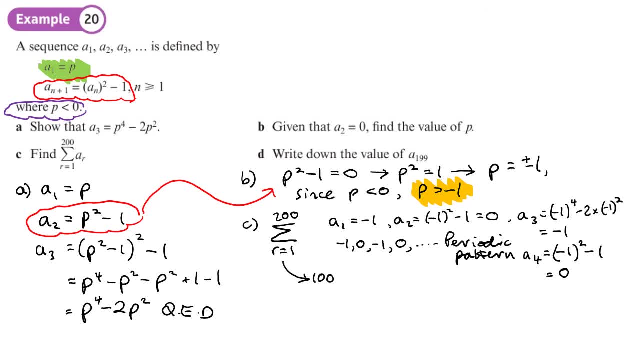 with this. I'm going to have a hundred terms of zeros, so I'm going to have a hundred zeros and I'm also going to have a hundred negative ones. in this pattern that goes: one zero, one zero. so what's the sum of that? well, it's just negative. 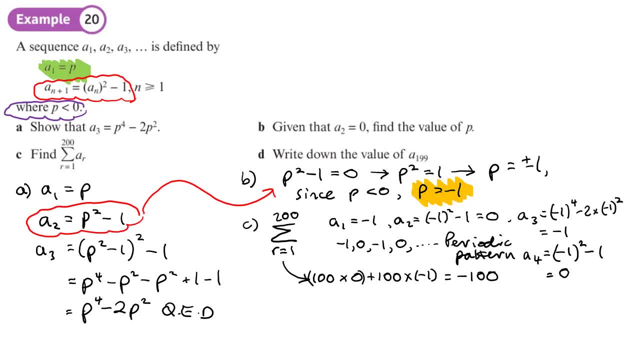 a hundred. so I didn't really need to do any working as such for that. I just needed to realize that I could have saved myself some time and I could have done better than that. so I need to write down the term and then I can write it down and so on, so I could're gonna empty theitsu didn't work, stick I would. 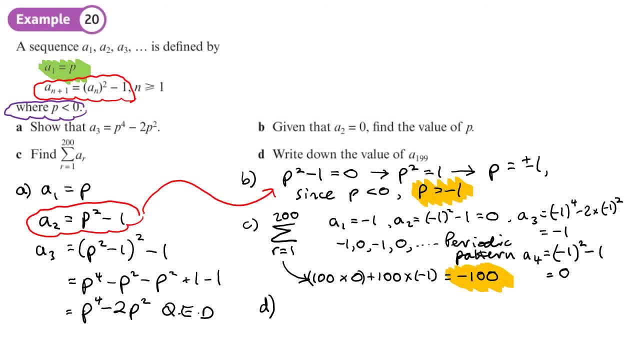 like to Wenner, and we're just going to remove this permanent variable down here, and then I think I need to do my ¿me que focuses the a, 3, a, 5 and so on. I'll say 5, I said 5, I wrote down 3. not sure what that's about. 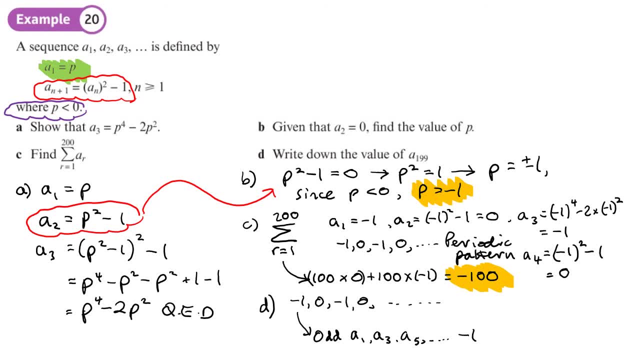 they're all negative. 1, yeah, where that little subscript is odd number, where that little subscript is an even number. so a 2, a 4, a 6, they're all going to be zeros. now we've got a subscript with an odd number: 1, 9, 9. so that's going to be. 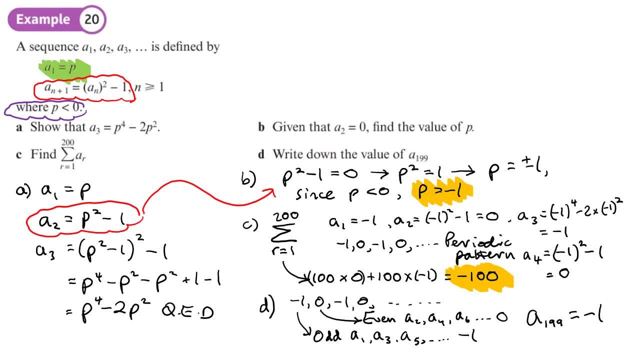 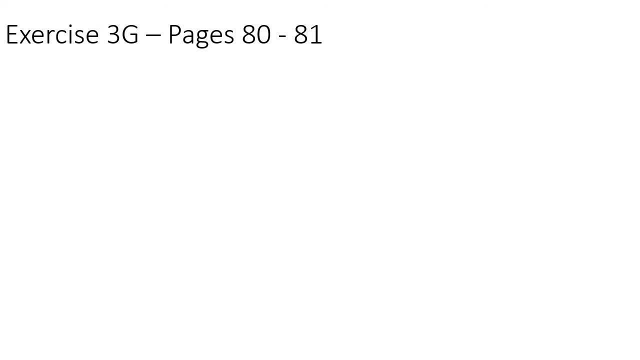 negative 1, so we just write that down. negative 1 is no real working that we have to do for that. so let's just highlight that now you should be in a position where you can do exercise 3g on pages 80 to 81. 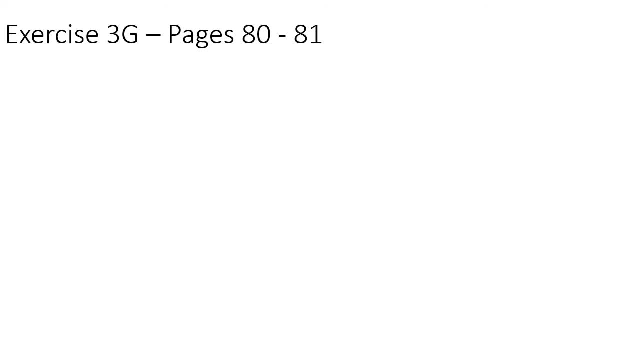 so you want to be in a position where you can do exercise 3g on pages 80 to 81. so you want to be in a position where you can do exercise 3g on pages 80 to 81. so you want to pause it now, have a go at that. but this video continues because there is 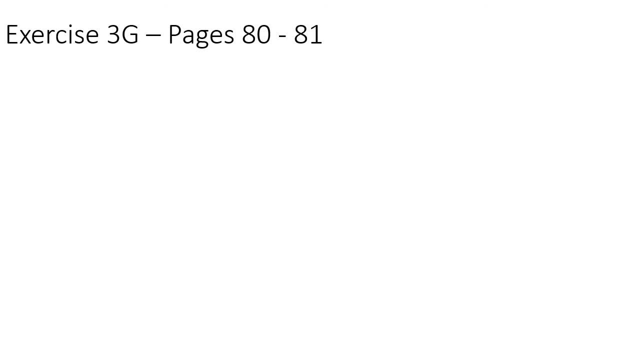 more in this section, which we're going to continue and have a look at. this is the second part of this section and I think it's not pretty straightforward. so we're looking at increasing sequences, decreasing sequences and periodic sequences. so let's start with increasing sequences. so I'm going to write the. 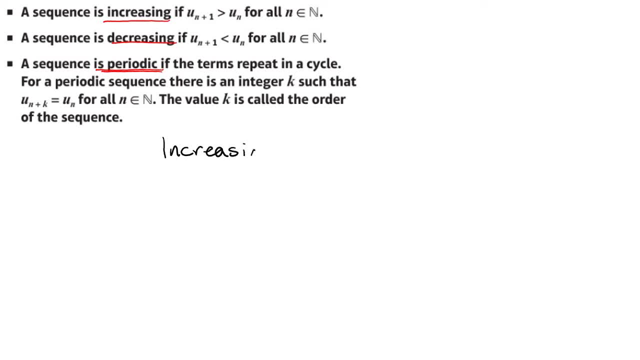 stuff at the top of my, my own words. if a sequence is increasing, then basically the next term. in a sequence which is basically u? n plus 1, the next term is always greater than the previous term. so that means it's always greater than u? n for an increase in sequence. if 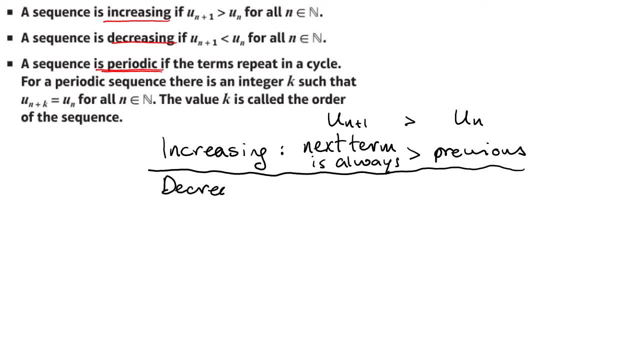 a sequence is decreasing, then the opposite it is true, and that is that u? n plus 1, which is the next term, the next term is always less than the previous term, so it's it's going down. each term is less than the last, so you u? n plus 1 is always less than u? n, so it's. 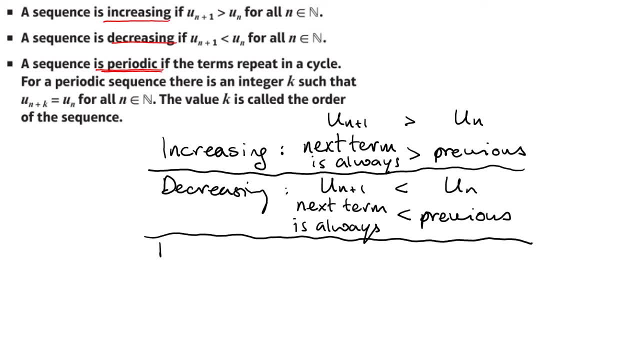 increasing, decreasing. now we have what we call periodic sequences. sometimes we- and this is where the terms go around in a cycle. the terms go round in a cycle, okay, and the should be really be a comma- the length of the cycle. the cycle is called its period. so here's an. 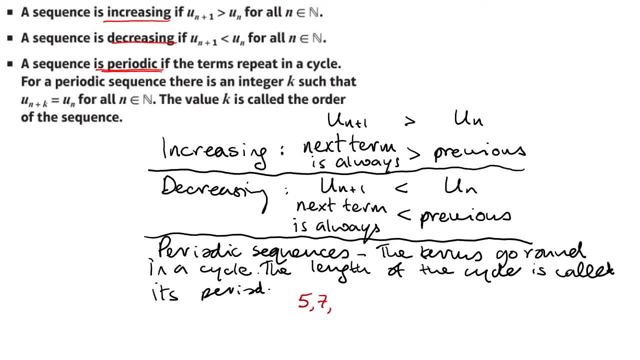 example, five, seven, three negative two, five, seven, three negative two and so on. this has a period of four because there are four digits or four numbers in that cycle before it repeats. so this has got a period of four and we know that, for example, if this is u1, u1 is going. 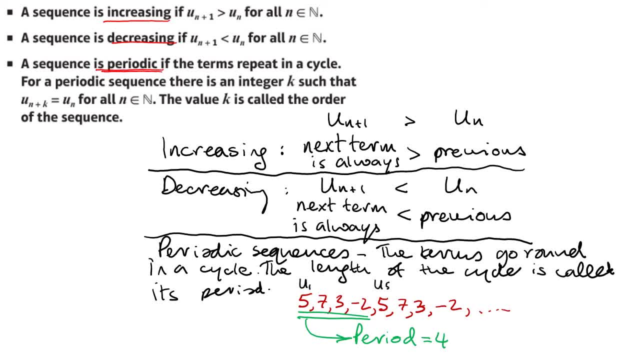 to be the same as u5 and then the same as u9. so if I add on the period to the first one, and then the second one, and then the third one, and then the fourth one and then the fifth term. so if I add on the period to that subscript I get the next term. that's the same if I add on. 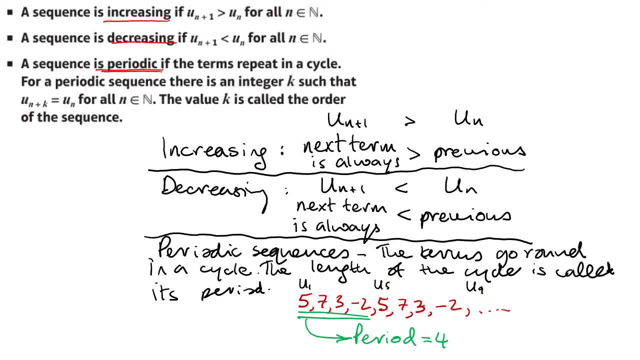 the period to that subscript, I get the next one that's the same. so, for example, at u3- now which other term is going to be the same as that? well, I add the period of four onto that subscript, so that should be used. seven, which is that one there, and then add that period on again. the next one. 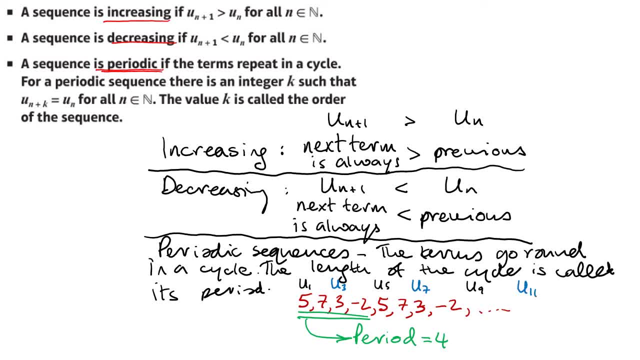 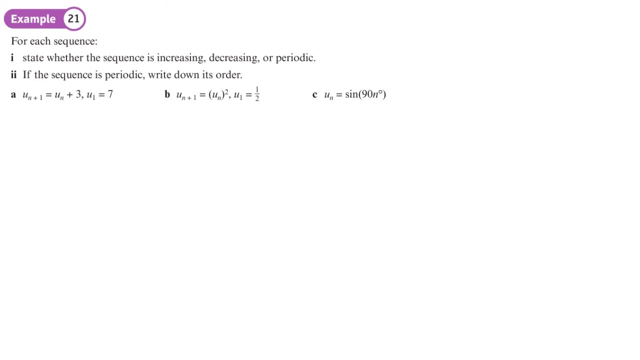 will be you eleven. that's what this bit down here is all about. yeah, basically saying, if you you've got a term, if you add on the period to it, you get the next term which is the same as it. which is sort of what we've basically done down here. okay, each one of these, we just need to state: 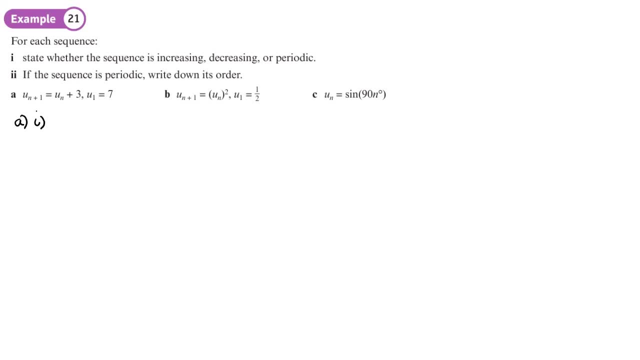 with her there and state just means. you don't really need to do any working, you just need to look at it and decide whether it's increasing or decreasing. so the first one, part one is increasing because we start with seven. you add for you had for, you had three, so I can see that's. 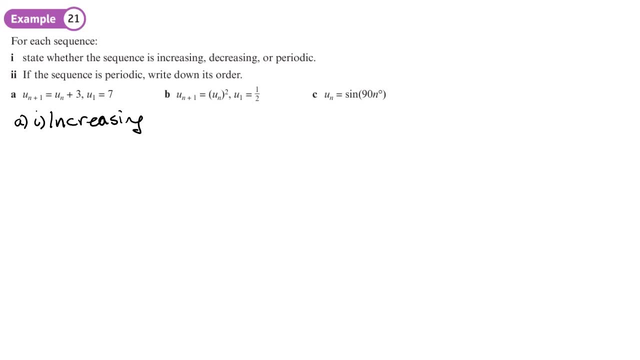 increasing. the second part of question: if the series series is periodic, that doesn't. it's not pickable, it's not periodic. and I write Part B- let's see what's going on here, right? so we start with our half, then we square it. yeah, quarter you square it, you get one. sixteenth, we square again. 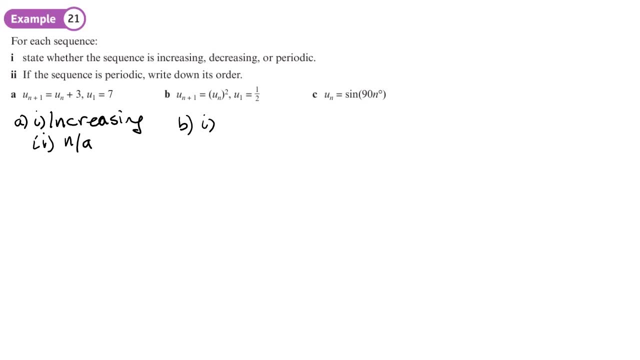 you one over two, five, six, I think, something like that. so it's decreasing. each fraction is smaller than than the last, so we don't need to write terms out. we can work this out in our heads. so this is a decreasing sequence. again, part two of the question is not applicable because it's not periodic. I reckon C is. 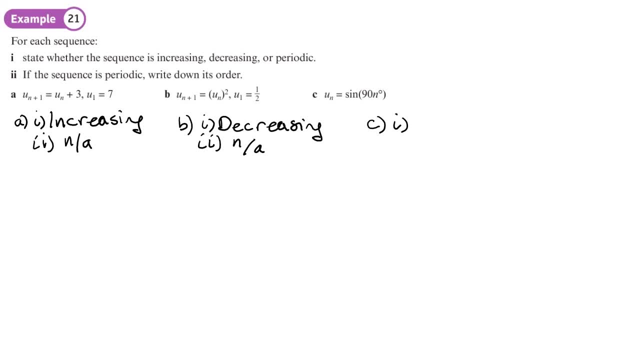 periodic. that's the one we haven't used yet. so this is basically what's happening to sine every 90 degrees. so sine at 90 is going to be 0, then I'll just write it down. so sine 90- might be worth writing this down- is 0 then when. 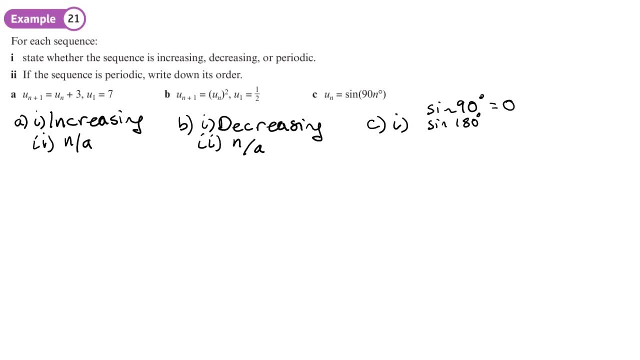 n is 2, it's sine 180, and sine 180 is 0 of 180 is 0. sorry. sine 90 is 1. what am I talking about? why didn't anyone say anything? so sine 90 is 1, another 90 sine 270. so this is 3 times 90. that's going. 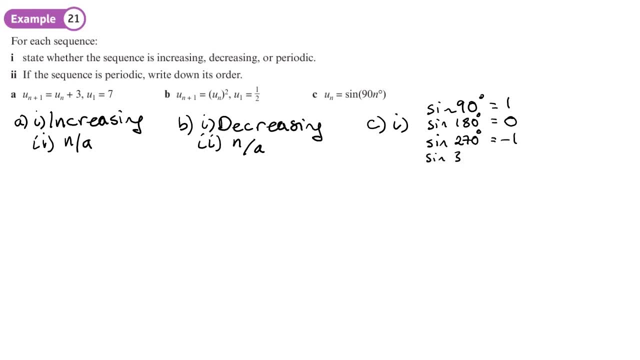 to be negative: 1 sine 360. this is going to be 0 again, and then we're going to get back to 1. so this is a cycle that goes 1: 0 negative, 1 0, 1 0 negative, 1 0. so